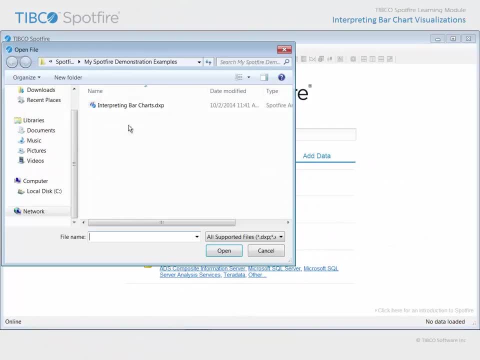 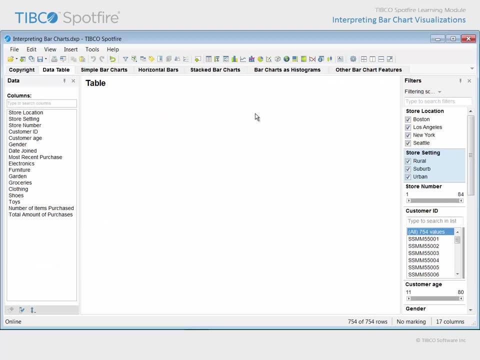 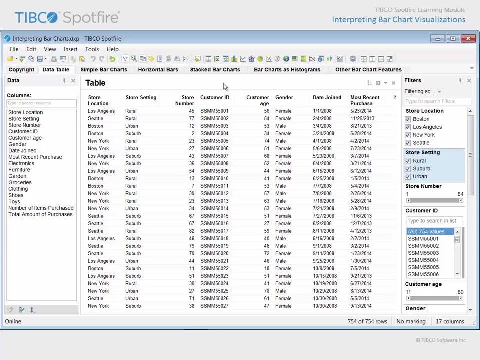 Use Open File in order to navigate to the configured Spotfire analysis document with Interpreting Bar Charts in the title. Click Open and agree to the terms and conditions of use. The data table which supports this analysis contains purchase data for customers shopping at a Mega Mart chain of department stores. 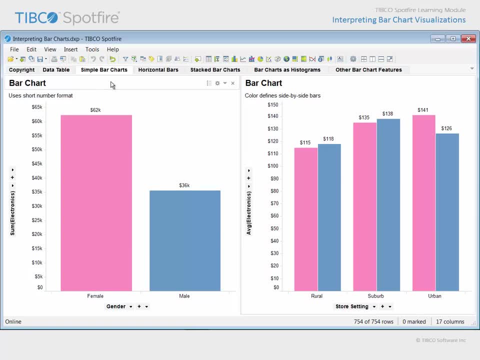 On this page, two simple bar charts have been configured. The bar chart on the left compares the total electronics purchase amounts made by men versus women, while the bar chart on the right displays the average electronics purchase amount made by men versus women at each store setting. 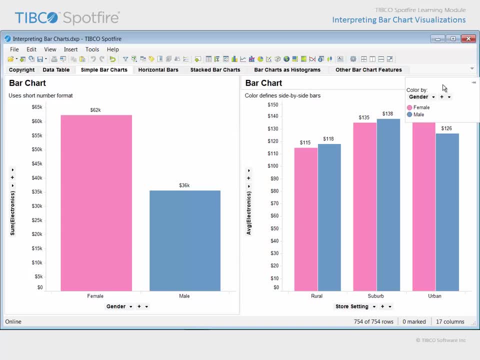 and even though both bar charts have gender applied as the color-by variable, it is important to note that the gender in this bar chart actually defines a grouping of values which is distinct and separate from the variable applied to the category axis, thus resulting in side-by-side bars and allowing for an easy comparison of gender-based electronics purchases in each store setting. 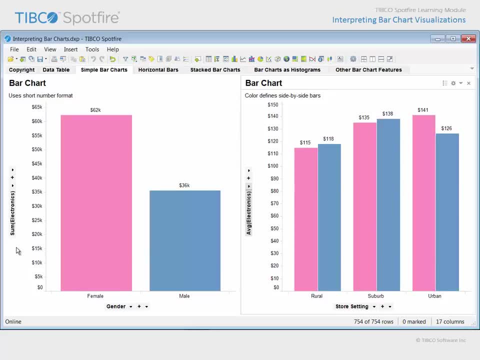 Also note that the value axis references the same column of data in each visualization, but the aggregation of values from that column is different. Also note that the value axis references the same column of data in each visualization, but the aggregation of values from that column is different in each chart. 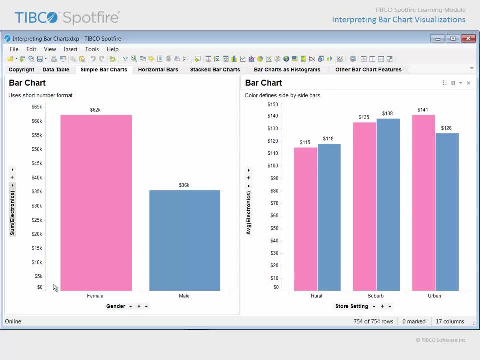 a sum in one and an average in the other, And because the sum of electronics purchases for each gender results in rather large values, the format applied to the numbers displayed in this bar chart: substitute a letter K for the three trailing zeros, which would make this bar height read $36,000. 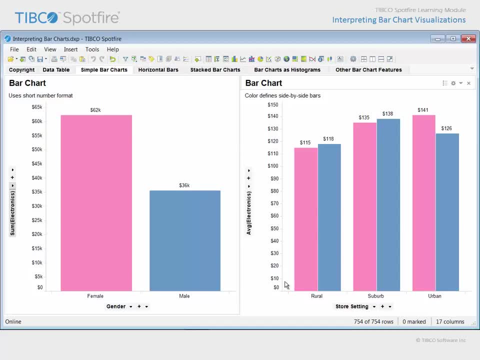 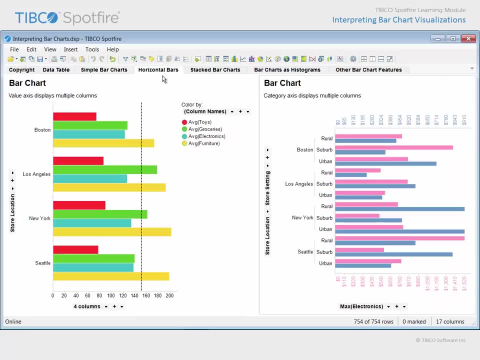 The numbers in this bar chart are not large enough to be suitable for that type of short number format, indicating that numbers may be formatted differently in different visualizations On the next page. both bar charts have been configured to display horizontal bars. This bar chart compares average purchase amounts across four different departments in each store location. 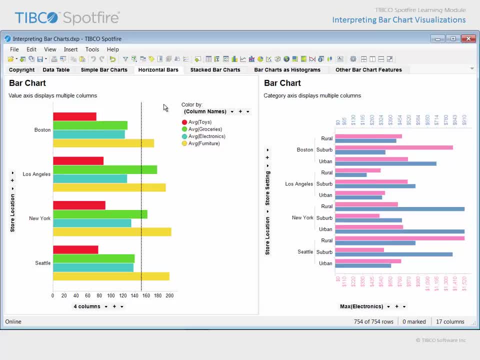 Each department is represented by a separate column of data in the underlying data table. therefore, each of those four columns has been assigned to the value axis and the color by variable has been set to group data into bars of different colors based upon each column name. 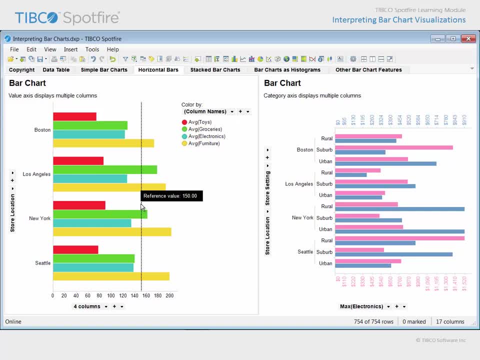 You will also notice that a reference line has been drawn at a fixed value with a fixed position of 150. in order to aid in the comparison across all locations, This bar chart has been configured with multiple columns assigned to the category axis. Consequently, the bars are split first by major store location, then split again by the store setting, thus creating a hierarchy. 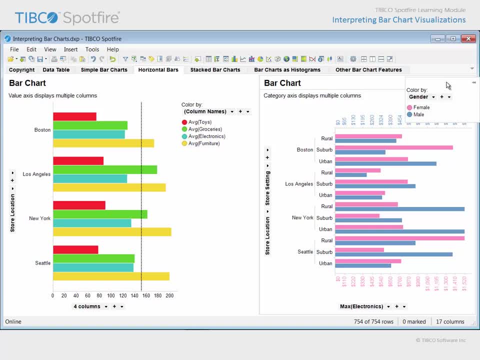 The final level of the hierarchical split is defined by the color by variable, which groups the data into separate bars for each gender. You may have noticed that there are two scales displayed on this bar chart: one colored pink, the other blue. This is because the values from each gender have been set to define their range based upon separate scales. 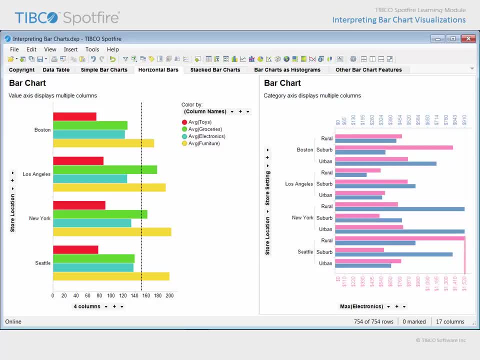 where the upper range limit is defined by the longest bar for that gender. Therefore, relative comparisons of maximum purchase amounts made by men versus women are readily available in each category, but a comparison of absolute values is extremely cumbersome in a bar chart configured in this manner. 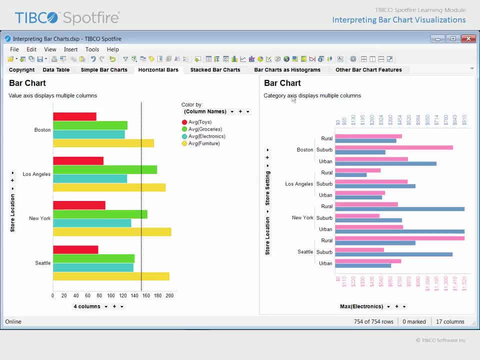 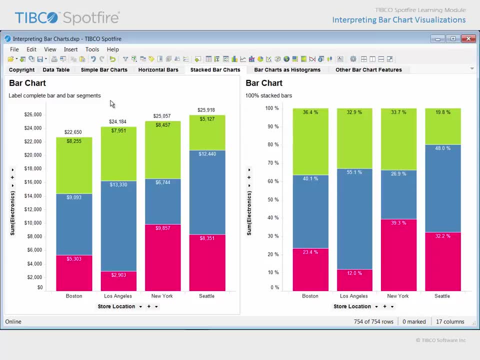 While these bar charts use color to define side-by-side bars, the bar charts on this page use color to define the color of the bar chart. This bar chart displays absolute total electronics purchase amounts made at each major store location as the overall bar height. 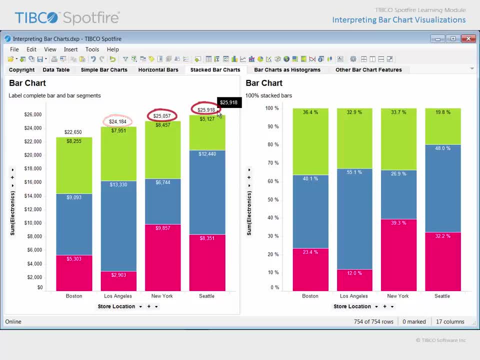 and you can see that this label indicates the value for the complete bar. Each bar is also subdivided by the store setting where the purchase was made, and labels showing the amount represented by each of those bar segments has been displayed. The bar chart on the right shows exactly the same data. 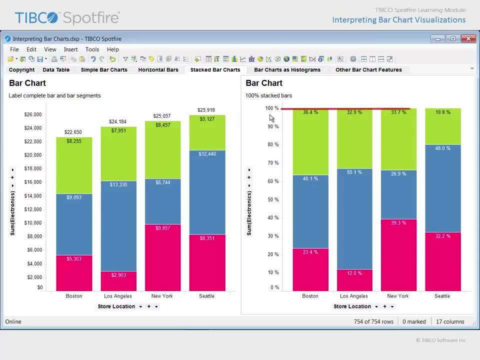 However, the overall bars have been normalized by the bar chart. You can see they're now being normalized to a height of 100%. Again, while absolute comparisons are no longer possible, relative comparisons of the percent contribution of stores from each setting toward that location's total. 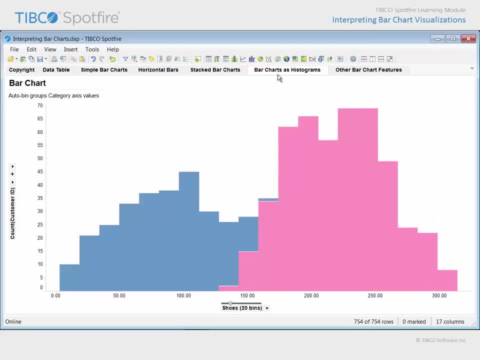 are now made available for comparison. On the next page, the bar chart visualization has been configured in an entirely different fashion. Here, the amount each customer has spent on shoes has been selected as the category axis. You can see that 20 bins have been derived from these values. 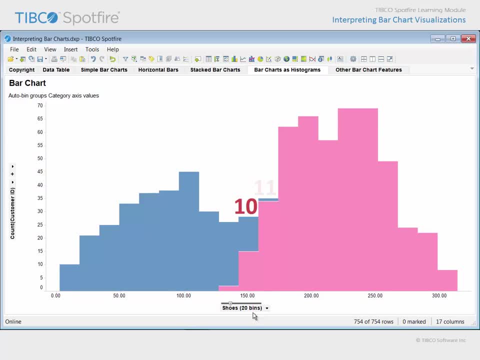 As you can see here, theность value沒有augen dengan plankton Ф не проверев means that the shoe purchase amounts have been grouped into 20 bins or purchase amount ranges in order to form 20 bars in this bar chart, And the value axis has been configured to count. 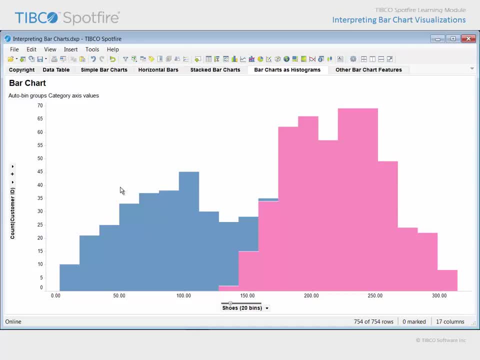 customers in each of those bins. Therefore, we can see how many customers made lower shoe purchase totals and how many customers made higher shoe purchase totals. Hopefully, it is immediately clear that this histogram represents two distinct populations of shoe purchasers, And it just so. 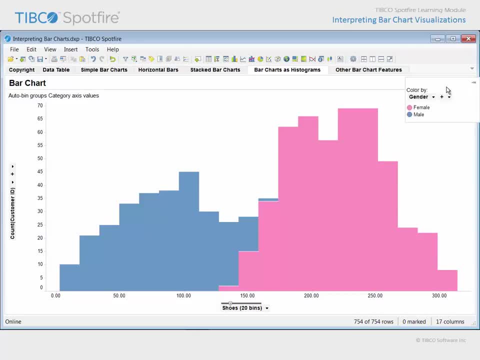 happens that each population is aligned with a gender indicated by color. If you would prefer to change the number of bars or groupings of customers in an attempt to achieve a better resolution of these distribution patterns, you can slide this bin slider to the right, As we do. 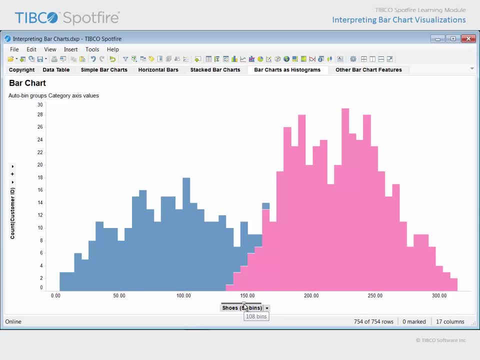 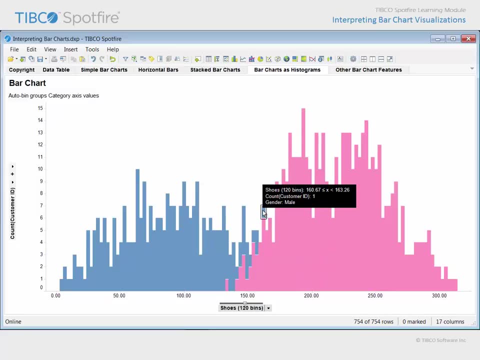 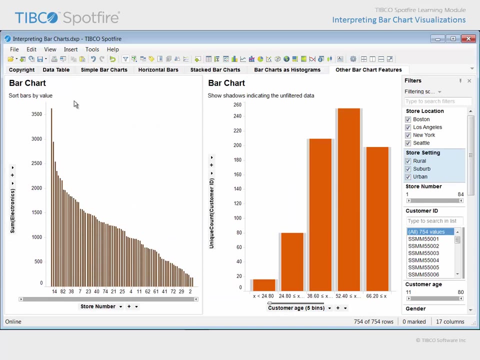 it becomes clear that, while the distribution is bimodal, the two populations are not completely separated And outlying customers of each gender occupy an overlapping region of shoe purchase amounts in the center of the overall range. On the final page of this configured analysis, a traditional bar chart has been created, which 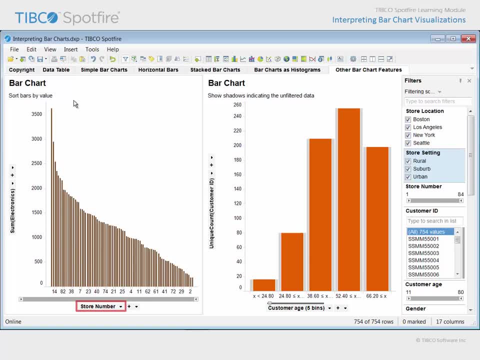 shows the total electronics purchase amounts made at each store, resulting in 84 bars. In order to make this chart easier to interpret, those 84 bars have been sorted from tallest to shortest, going from left to right. In addition, a zoom slider has been added which allows us to zoom. 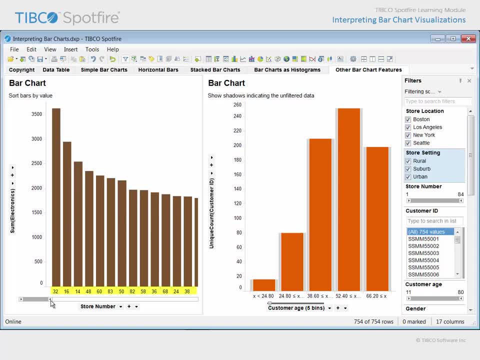 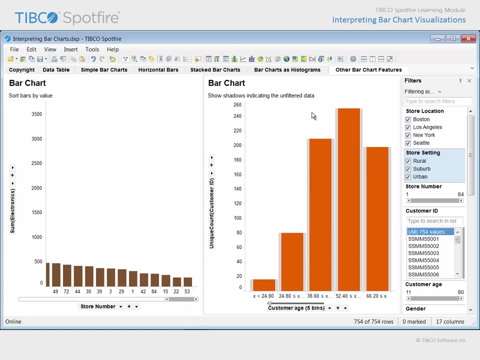 in on the taller bars such that we can read the individual store number values. In addition, we could grab in the middle of the sized slider's gray region and drag in the direction of the shorter bars in order to examine adjacent store number values along the way. This bar chart has been configured as a 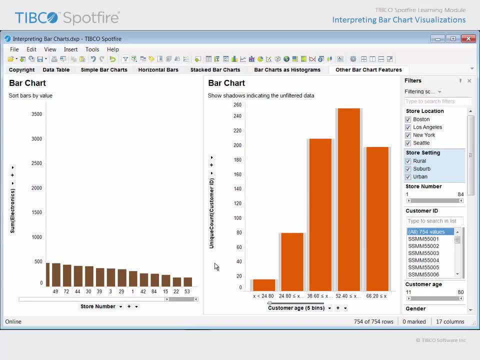 histogram and the count of customers is reflected in the height of each bar. Currently, all customers from the underlying data table are contributing to the height of each bar. However, if we use the filters panel to remove Los Angeles customers from the bar chart, you can see that the visualization 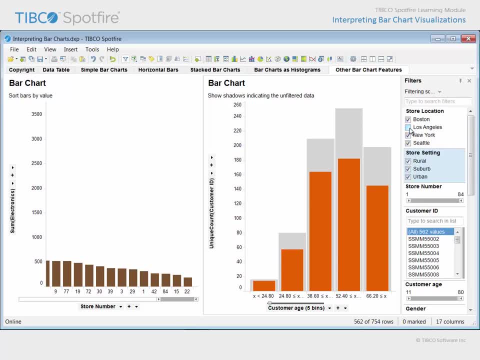 has been configured to show a shadow indicating the bar chart has been configured to show a shadow. So while subsequent filtering to remove all suburban customers from the visualization will further decrease the height of the orange bars, the height of the shadows will continue to display. 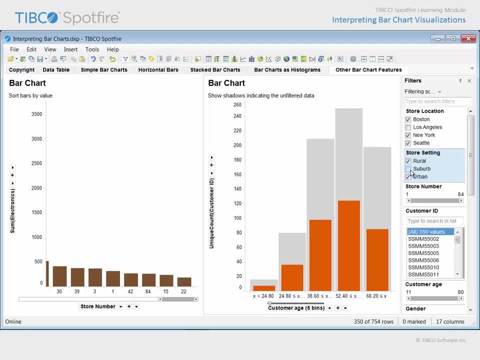 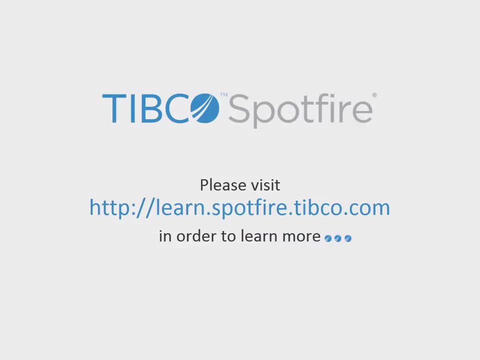 the age distribution pattern of the unfiltered customers from the underlying data table. In addition, the set of the two bars also indicates that the ratio of the price, the cost and the number of customers are recorded is measured and that the number of customers are considered.